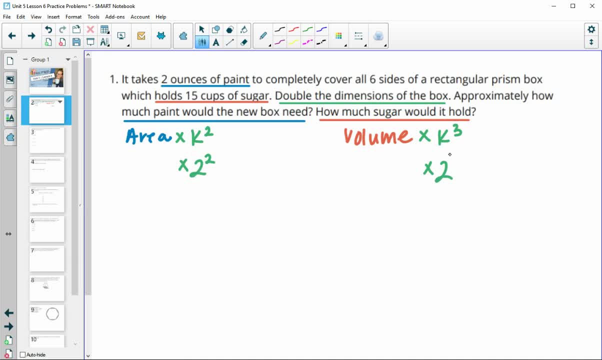 So we're going to multiply the area by two squared And we're going to multiply the volume by two cubed, So our original area- again we're talking paint, And so the original amount of paint was two ounces of paint. So we're going to do that here. 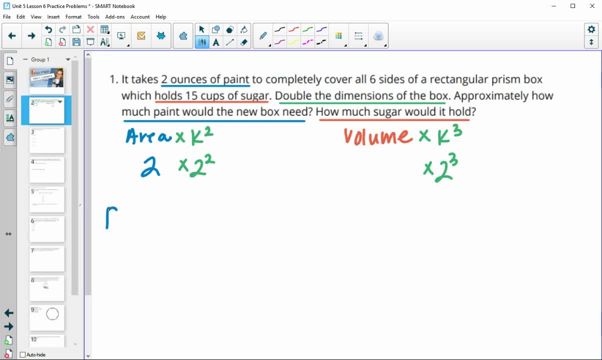 two times two squared, Okay. So the new amount of paint needed would be two times four or eight ounces. Then for the volume: okay, our original volume was 15 cups, So we had 15 cups of sugar. So then we're now going to be able to fit in 15 times two cubed, or 15 times eight. 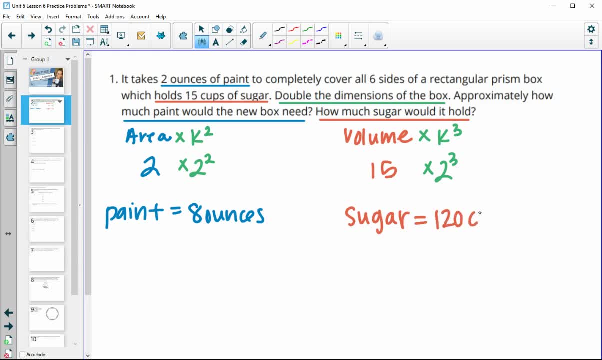 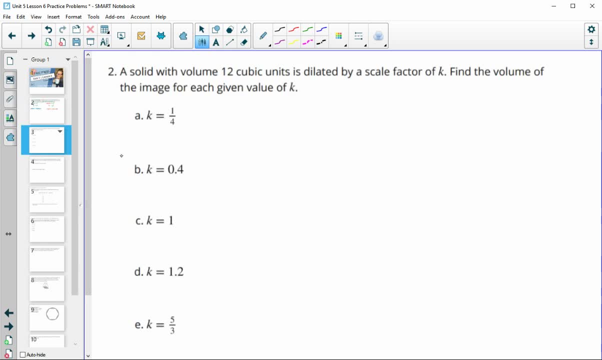 which is 120 cups of sugar. in our new box, Number two, we have a solid with a volume of 12 units, So we've got volume given to us here. And then we have a solid with a volume of 12 units, So we've got volume given to us here. 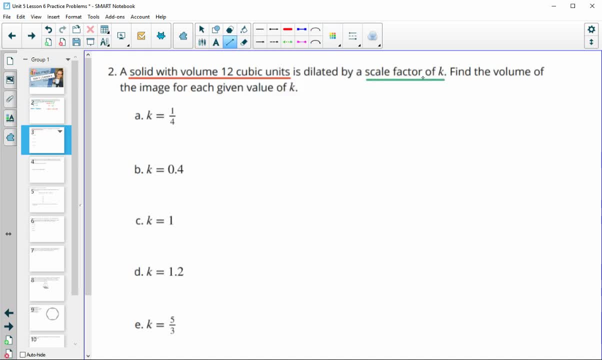 And then we have a solid with a volume of 12 units. So we've got volume given to us here And then they're dilating by each of the scale factors given and we want to come up with the new volume. Okay, So our original volume is 12.. So we're going to take 12 times. 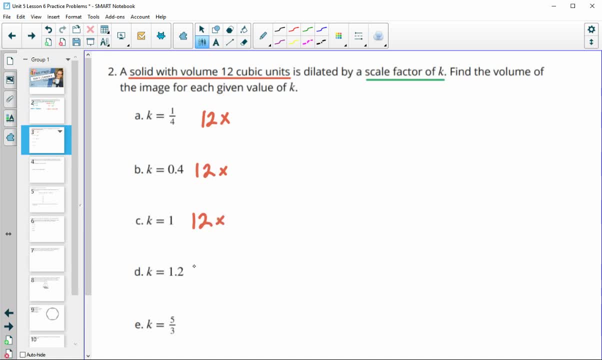 each of these scale factors. And when we're dealing with volume, remember that we multiply by our K cubed. Okay, So volume needs us to multiply by K cubed, So we're going to be multiplying by, in this first one, one fourth cubed or in this next one, 0.4 cubed times one cubed times 1.2 cubed. 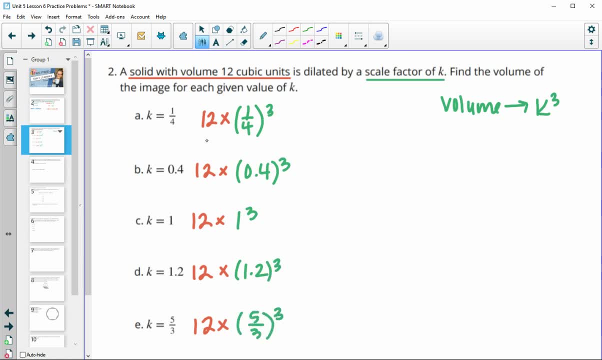 and times five thirds cubed. So the original volume times the scale factor cubed. And so when we do this for this one, we get 0.1875, and then cubic units For volume. Okay, for this next one, when we do 12 times 0.4 cubed, we're going to get 0.768 units. 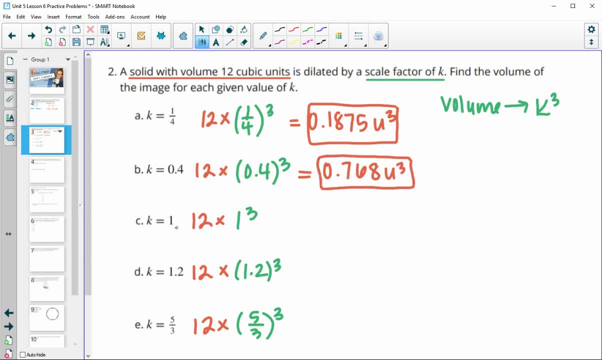 cubed. Scale factor of one doesn't change anything, So we're just going to continue to have 12 units cubed. Multiply 12 times 1.3, or sorry, 1.2 cubed, And we'll get 20.736 units cubed. And this scale factor was larger than one, So our volume went up. 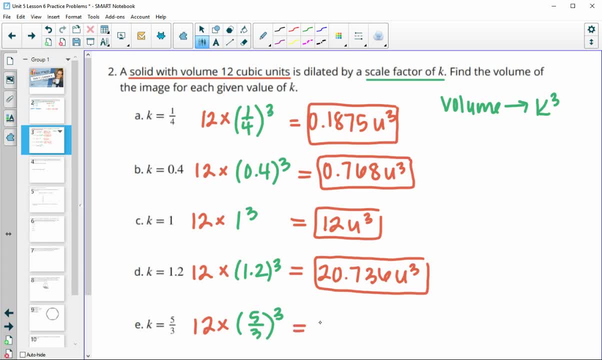 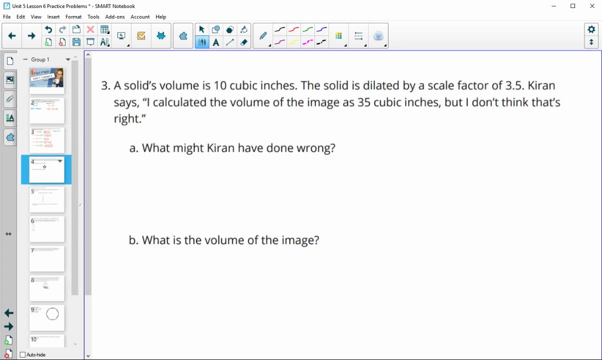 versus these other ones have gone down, And then this is larger than one also, So this one's going to get bigger, And so when we multiply 12 times five thirds cubed, we get 55.56 units cubed for our new volume, Number three. 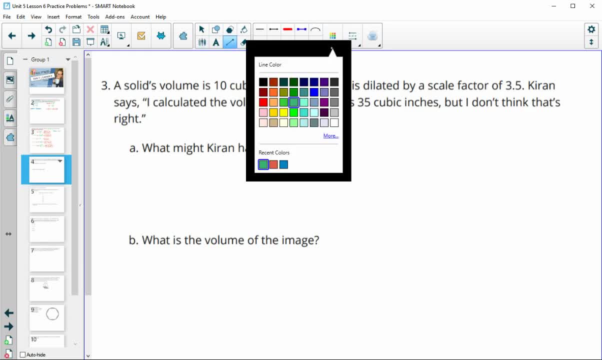 a solid's volume is 10 cubic units And the solid is dilated by a scale factor of 3.5.. Kieran says I calculated the volume of the image to be 35 cubic units, but I don't think that's right. What might? 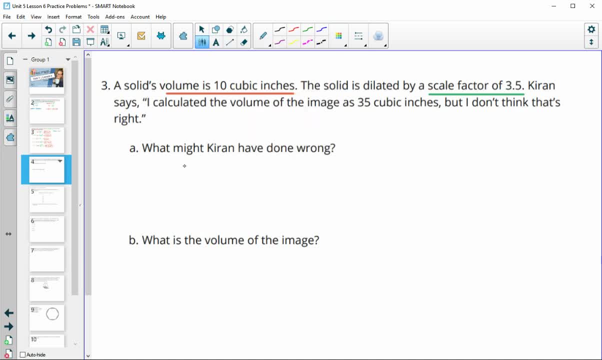 he have done. So it looks like Kieran took the original volume 10. And then when he multiplied, he multiplied by the scale factor of 3.5, because 10 times 3.5 does give us 35. And so when he was using 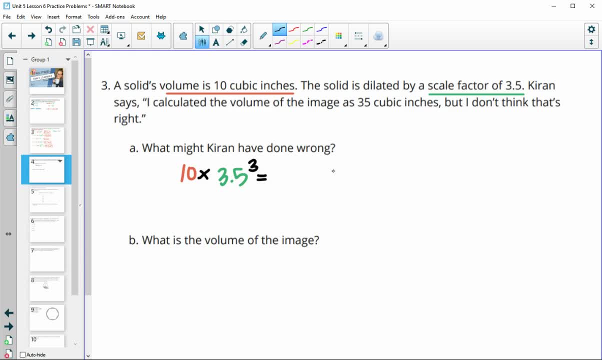 volume he should've been multiplying by this three point five cubed, So he multiplied by K instead of K? cubed, And so then, what would this volume be? if we did do 10 times three point five cubed, we would get our new volume as 428.75 inches cubed. 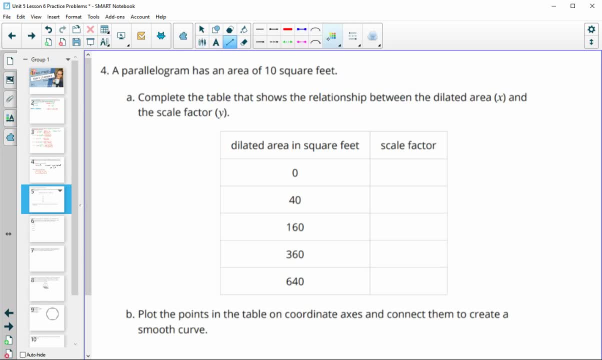 Number four: a parallelogram has an area of 10 square feet. Complete the table that shows the relationship between the dilated area, which is our x, and then the scale factor that would have produced it. So remember when we're doing area. 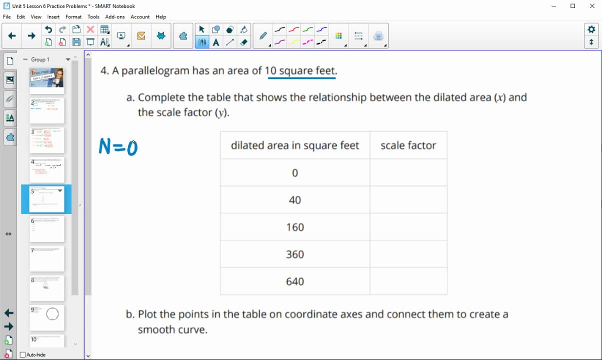 so our new area would equal our original area times k squared. So we're trying to solve. remember that the scale factor is k, so I'm going to take and divide by the original area. so that's going to give me new. divided by original, equals your k squared. 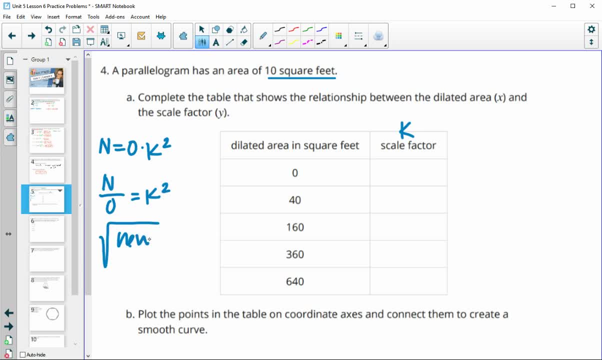 Then we're going to end up having to square root this. so we'll square root the new divided by the original and that's going to give us our k value. So we would do zero our new divided by the original. 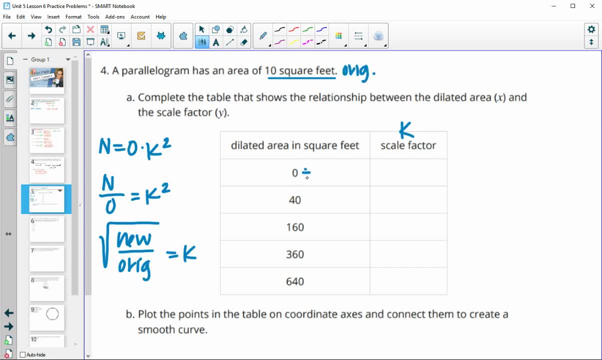 So remember, this is the original. So zero divided by 10, which is zero, and then the square root of that is zero. 40 divided by the original gives us four, and then we would square that and find out that our scale factor was two. 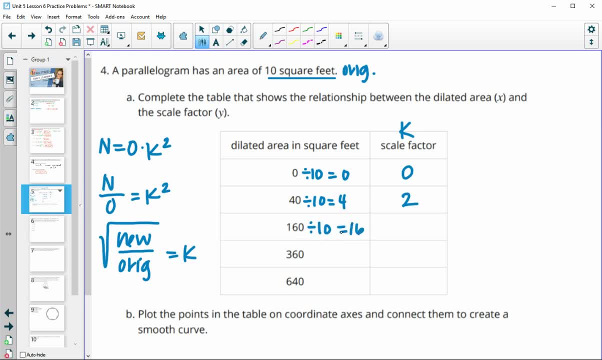 160 divided by 10 gives us 16 times bigger. so then we'll square root that and get four. Divide by 10 here gives us 36,. square root that and we'd get six Divide by 10, and we have that this area is 64 times bigger. 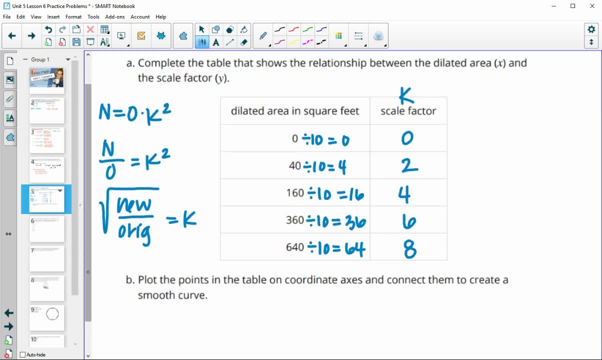 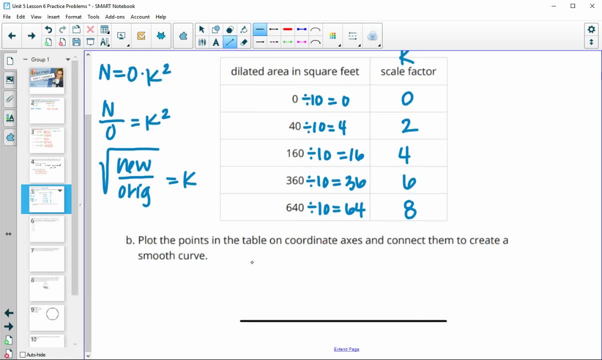 square root it and we would get eight for the scale factor. Then it wants us to plot these points on a coordinate axis and connect them to give us a smooth curve. So we need our x-axis to go up or, sorry, our y-axis to go up to eight. 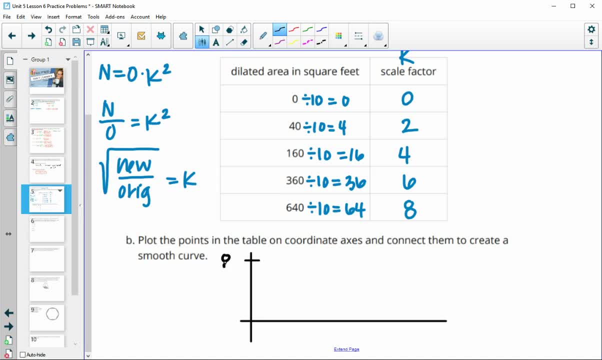 Okay, so I'll label this as eight, and then halfway between that would be four, So this would be two and this would be six. Then we need this axis to go up to like 640, so I'm going to put 600 here. 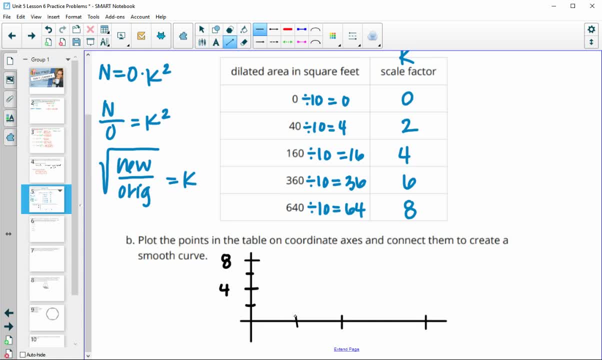 So halfway between that would be 300.. Halfway between that would be 150.. So we've got this at 600, this at 300, 150, and 450.. And so then we can start trying to plot these a little bit. 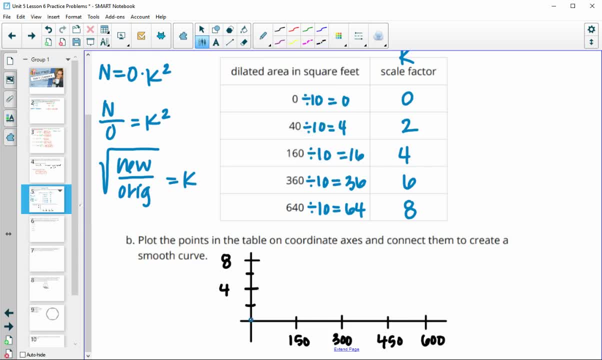 So at zero. we were at zero, Okay, at 40, which this is 150, so this is 75.. So 40, somewhere down here, that's at two, At 160, so just above 150, we were at four. 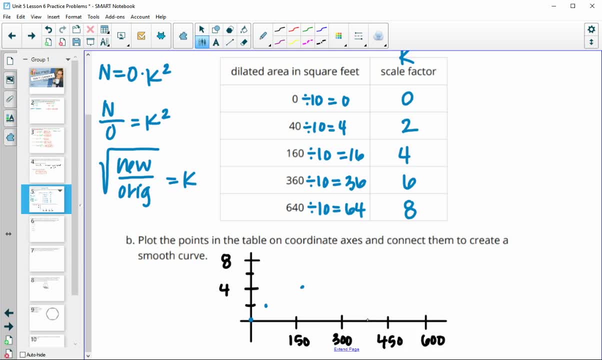 At 360, so here's 300, here's 450.. So 360, somewhere in the middle. here we were at six, And then at 640, we were at eight. So then just connecting that with a smooth curve. 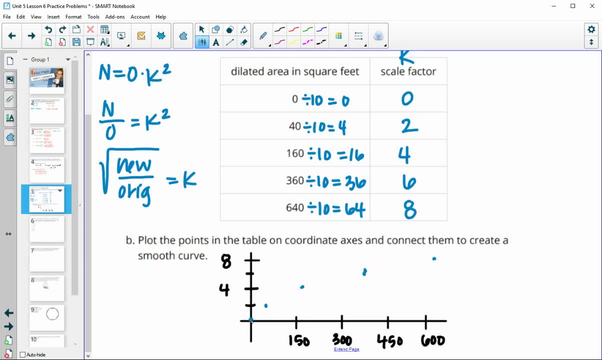 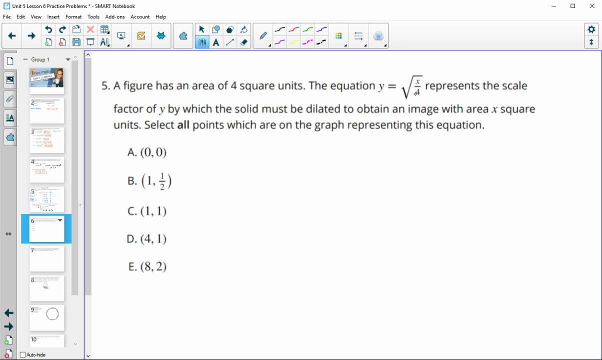 which. that wasn't very smooth. let's try again. So connecting that with a curve would give you something like that. All right, number five: a figure has an area of four square units. This equation represents the scale factor of y, by which the solid must be dilated to obtain an image with an area of x. 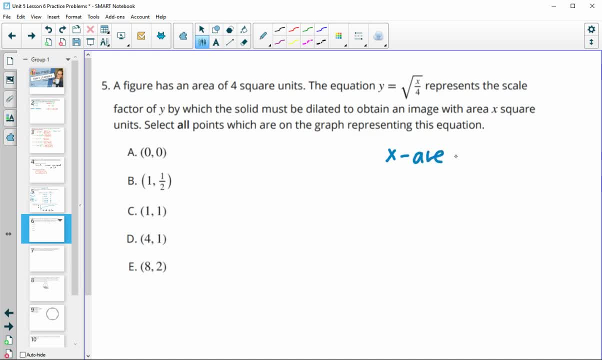 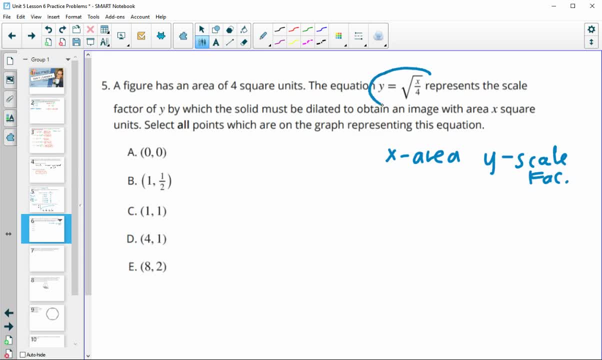 Select all points which are on the graph, So we just need to plug them into here and see if they equal out. So remember, the first one is x, the second one is y, So y equals zero. Does that equal the square root of x, which is zero, divided by four? 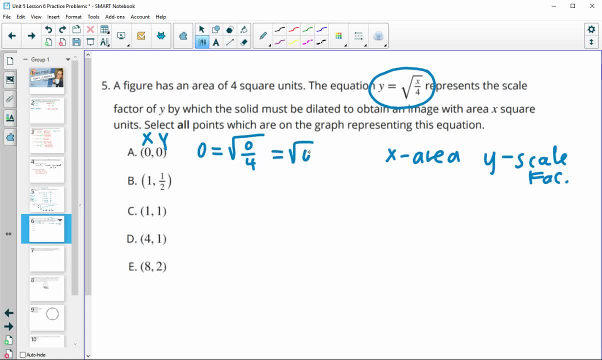 Zero divided by four is zero. The square root of zero is zero. So zero equals zero. So this one is good. Okay, this next one. the y value is one half. Does that equal the square root of the x, which is one over four? 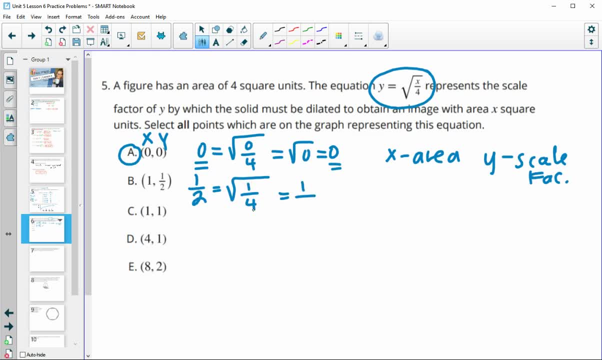 Okay, and for square roots, you square at the top, which is one, and you square at the bottom, So square root of four is two. One half equals one half, So this one is good. Okay, for this one. our y value is one. 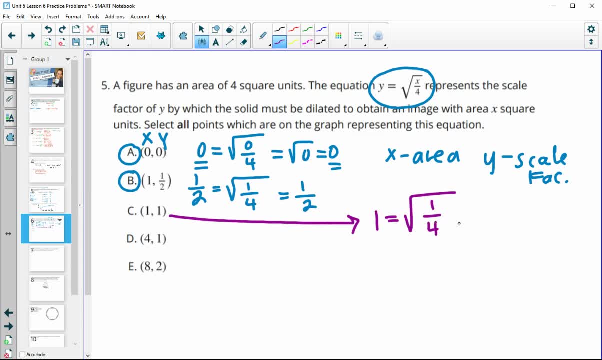 Our x value is one. So then we'll simplify this root here. Square root of one is one, Square root of four is two. One half does not equal one, So this one is bad. For this next one, our y value is one. 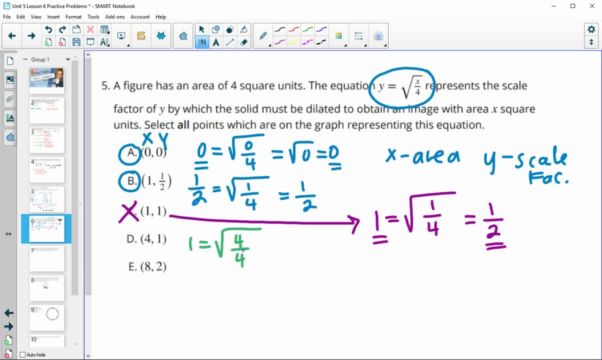 Our x value is four, So we get this, Okay. four over four is one, and the square root of one is one. One equals one, So this one is good. And then the final one: Okay, our y value is two. 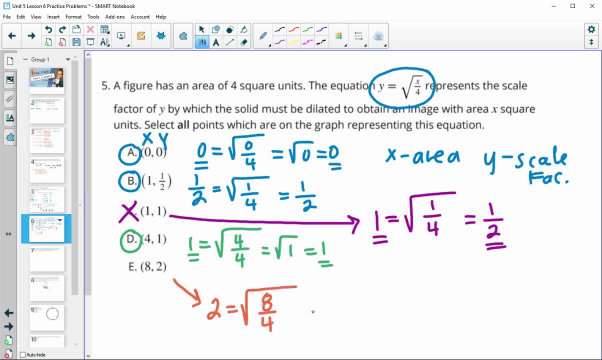 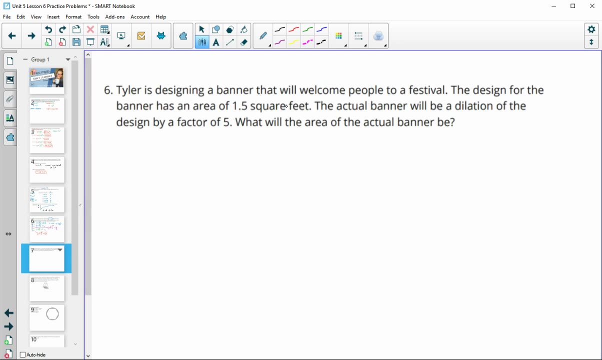 Our x value is eight, So eight divided by four, which is two, and the square root of two does not equal two, So this one would not be good. Six Tyler is designing a banner that will welcome people to a festival. The design for the banner has an area of 1.5.. 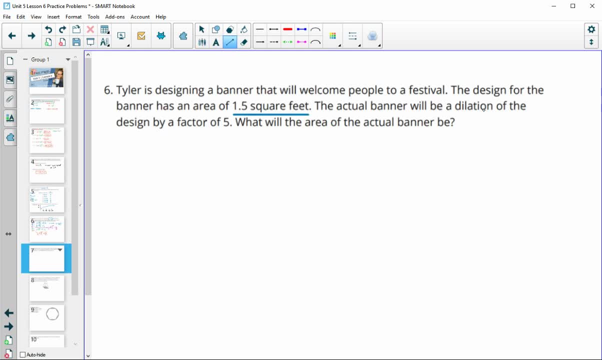 Square feet. The actual banner will be a dilation of this design by a scale factor of five. What will the area of the actual banner be? So remember that for this we'll do the original area 1.5, and then we'll multiply by the k value squared. since we're in area 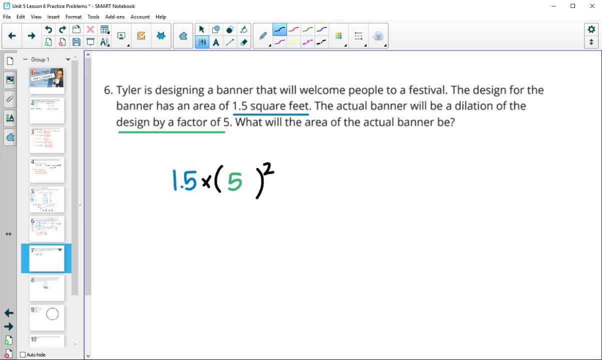 Okay, and the k value, or the scale factor, is five. Okay, Okay, Okay, Okay, Okay. when we do 1.5 times 5 squared, we'll get our new area of 37.5 feet squared. So that'll be the size. 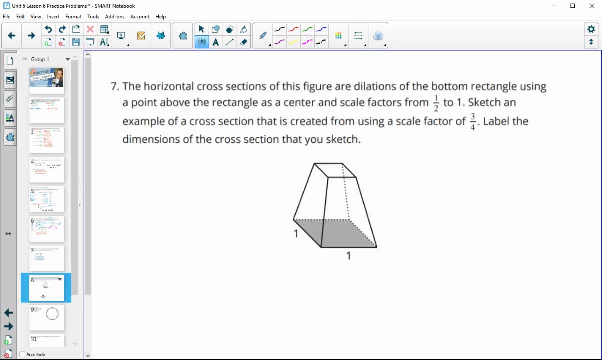 of the new banner, Number seven. the horizontal cross sections of this figures are dilations from the bottom rectangle using a point somewhere above it, And this has scale factors from one to one half. So this top, to get this top one, is a scale factor of one half. Sketch an example of a cross. 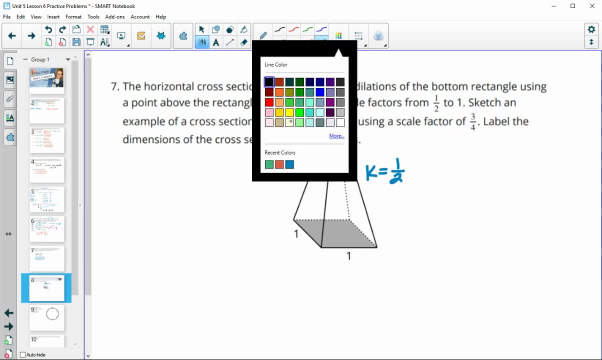 section that could be created using a scale factor of three fourths, And so three fourths, we know, is directly in the middle of so one half, which is in fourths, two fourths, and then one which in fourths is four, fourths, So three fourths is directly in the middle of three fourths. 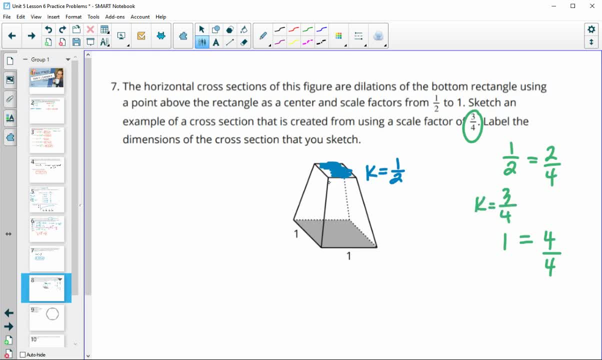 in the middle of that. So we want this K value to be directly halfway between this one half top and this one bottom. So then we'd want it to be kind of right here, And then the dimensions would be taking the original times your scale factor. So one times three fourths would be. 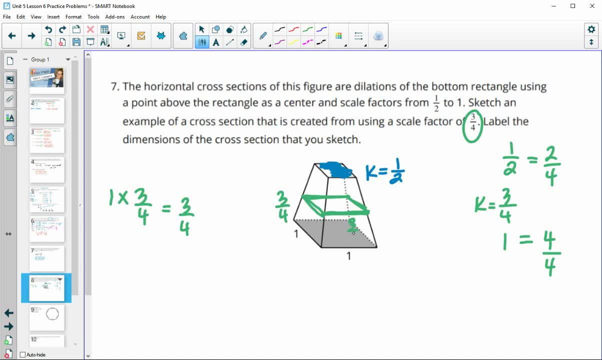 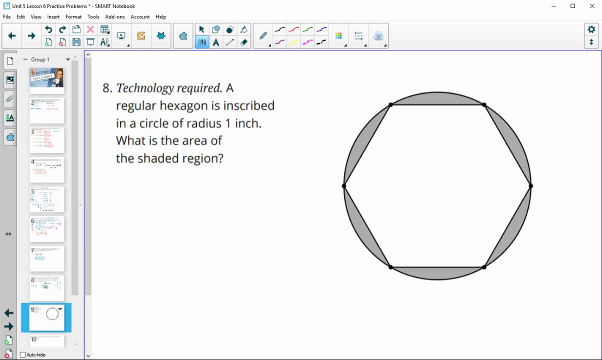 three fourths. So these would each be three fourths. All right, A regular hexagon can be inscribed in a circle with a radius of one. What is the area of the shaded region? So for this, we're going to first want to find the area of that circle. 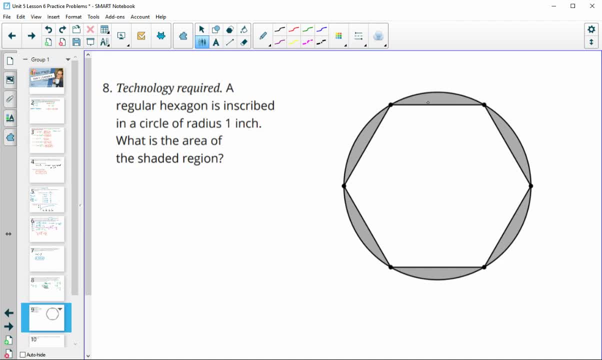 And then we'll find the area of the hexagon and just erase it out, The circle area. So for the area of the circle, remember that area is pi times the radius squared, And in this case they told us our radius is one. So the area of the circle is actually just 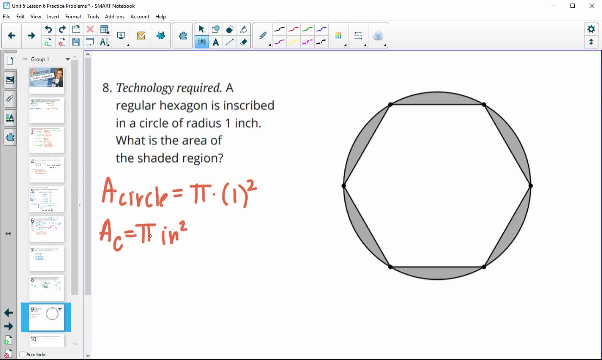 equal to pi inches squared. OK, so there's the area of our circle. Now we want to find the area of this hexagon. So for the hexagon area. remember that we can split this hexagon into a bunch of different areas. So we're going to find the area of the hexagon. So for the hexagon. 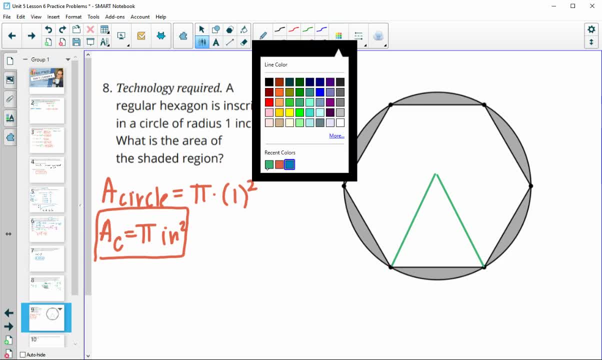 area. remember that we can split this hexagon into a bunch of triangles And then we're going to have to use trig. So the angle here, six of these will fit into this whole thing. So if we do 360 divided by six, we get 60 for this large angle here. Then we can go ahead and split this triangle. 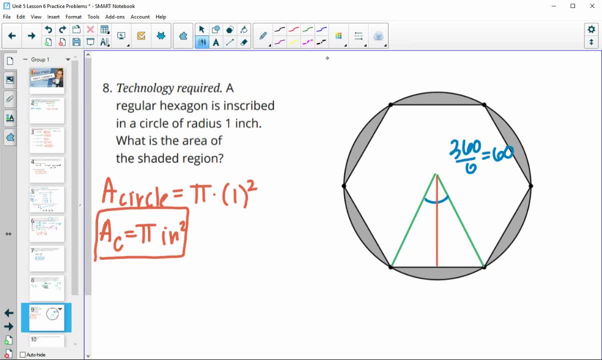 so we get the height, Since for area of a triangle we need to do base times height, And that would be half of this angle. So this is actually a 30 degree angle. And now, instead of using trig, we can actually use 30,, 60,, 90 formulas. So we know that this hypotenuse here. 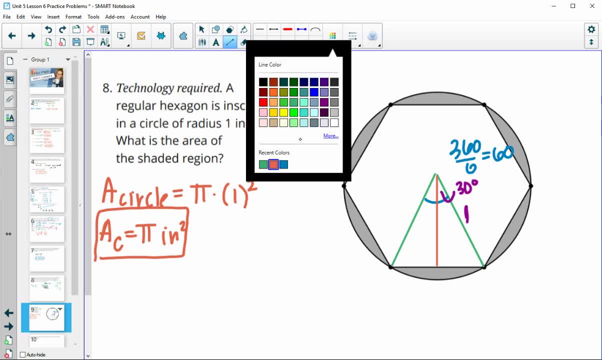 is one, since that's the same as the radius of the circle. So we can see. let me just get this drawn on here. So this is actually the same as the radius of the circle, So that length is one. And then, using 30,, 60,, 90 formulas, this would be the short side. So this would be half of the. 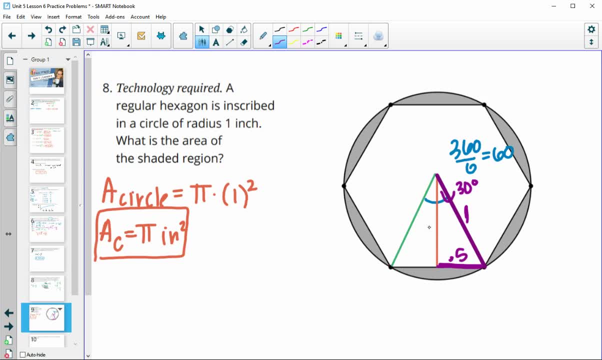 hypotenuse. So this would be 0.5.. And then this length would be the short side times the square root of three. So we would do 0.5 times the square root of three and that would give us 0.866. for 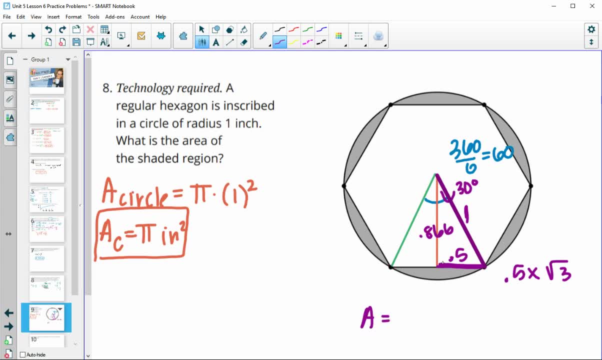 this height. So then we could find the area of this triangle, So this triangle by doing- and I'm just going to find the area of this whole triangle, So this length, right here is one, because this says 0.5.. So this would be 0.5.. So the base is going to be one times the height, which is 0.866.. 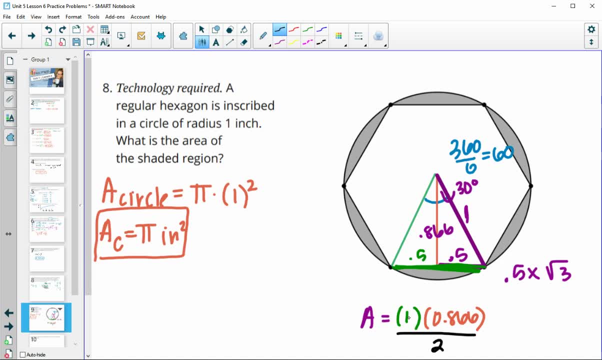 And then we would divide by two. So area of a triangle is base times height divided by two. So the area of this triangle is going to be 0.866 divided by two, or 0.433.. So that's the area of. 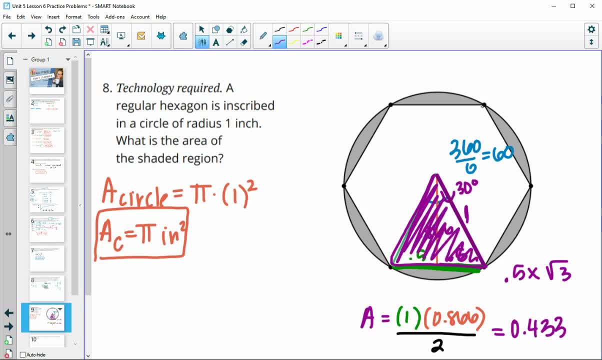 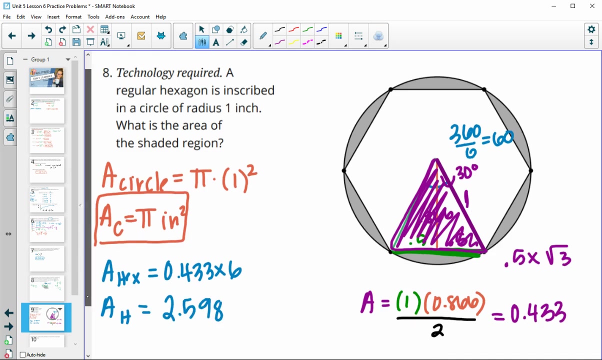 this triangle here, And then we know six of those fit into the hexagon. So the area of our hexagon is going to equal the area of that purple triangle times six. So the area of our hexagon is equal to 2.598.. So then to get the shaded region. 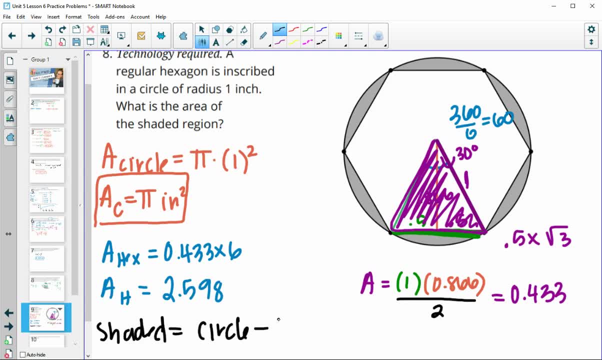 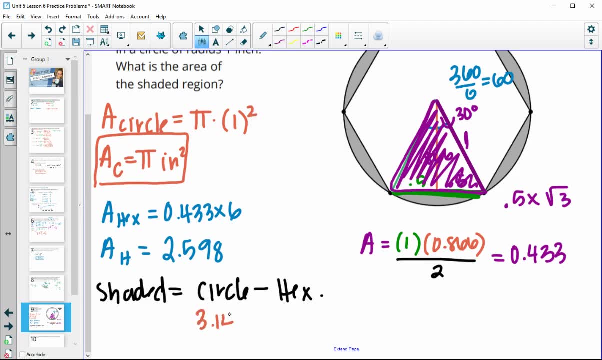 okay, we would take the circle and subtract the hexagon. So our circle is pi, which is 3.14159.. So 3.14159.. Whatever you, however far you want to go with that, And then minus the hexagon, which is 2.598. 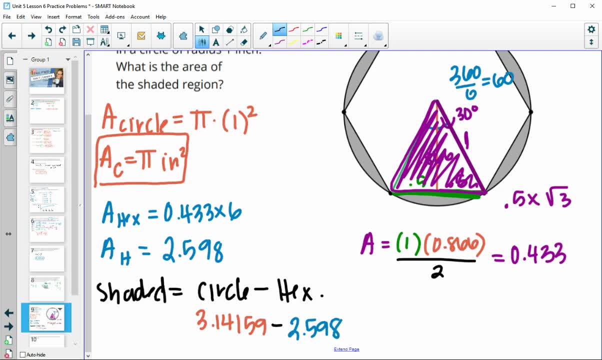 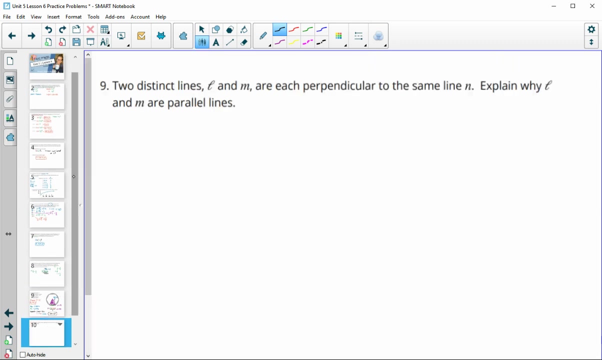 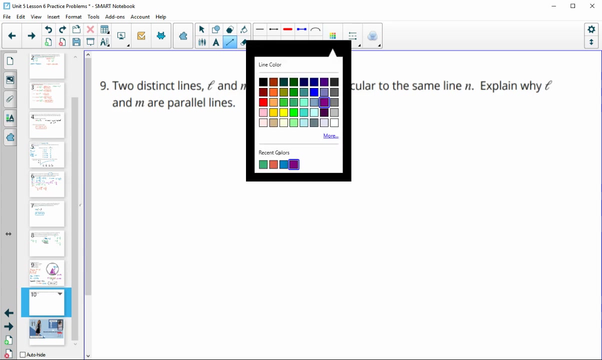 And so if we subtract that, we would get that the area of the shaded region is about 0.54.. And then inches squared. Okay, Alright. Then number nine says two distinct lines, l and m, are both perpendicular to the same line n. 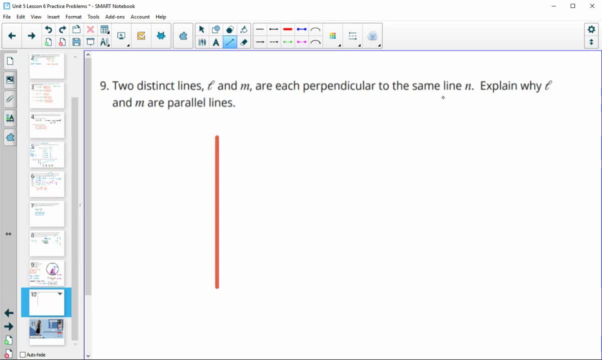 So let me draw an n first. So here's n, and then lines l and m are both perpendicular to it. So here's l and then here's m. They're both perpendicular to that line. Why are they parallel to each other? So we know that this is an irgendwie perpendicular line. So we know that this is a nearly perpendicular line to that line. Yeah, we know there is a parallel line to one other And then we just blanket that line of oen. So we know that this lines have to be woman's person, like.